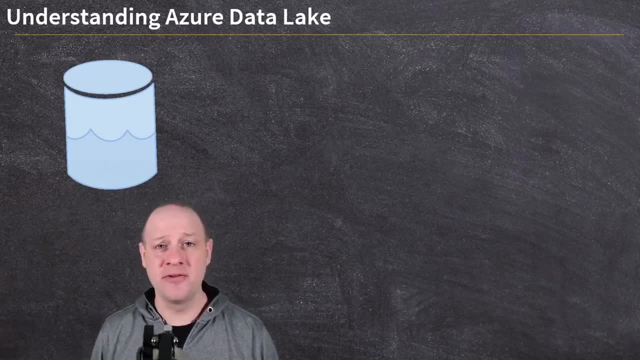 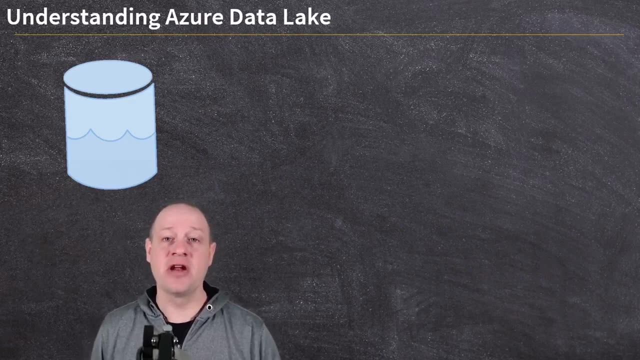 get data from Plus. we're getting data from everyone's tablets and cell phones and their cars. We're getting it from IOT devices. We're getting it from appliances. things like washing machines and refrigerators can now generate data. If you want to, you can collect a lot of data from 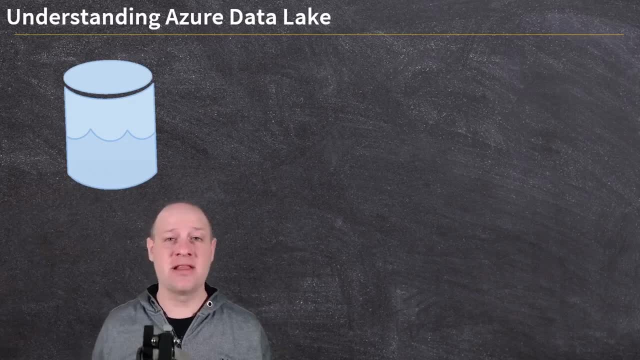 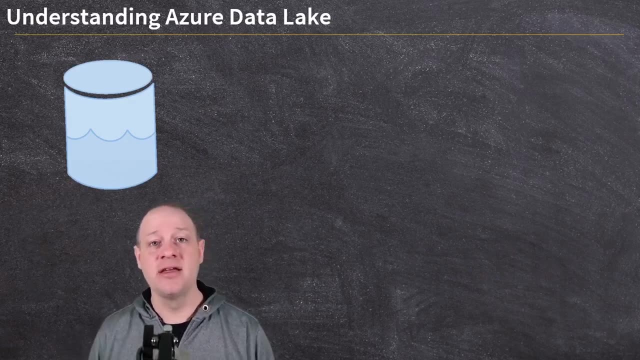 a lot of different sources that generated, in a lot of different ways, a lot of different rules and a lot of different structures. That's huge, That's a big deal And it's allowed us to make real change and real insight into our understanding of the world around us. The second thing is having 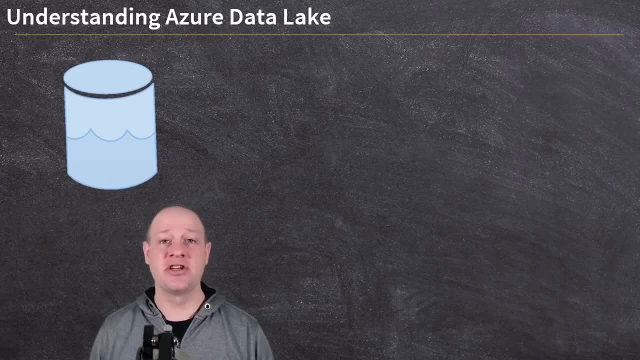 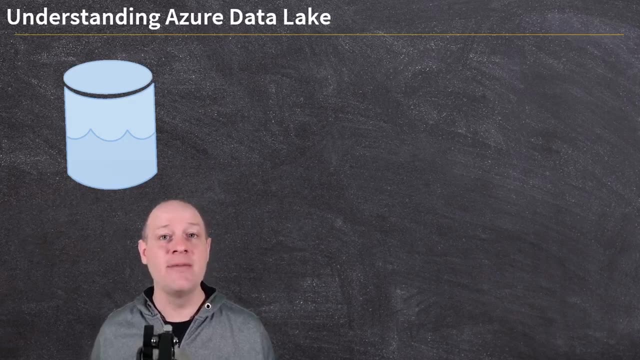 access to all that data means we need somewhere To store it, And that's the other thing that's really changed over the past 10 or 15 years: Cloud public providers offering us massive, near limitless storage capabilities at a fraction of the cost that it used to cost to well develop it ourself. So, with these two things combined, 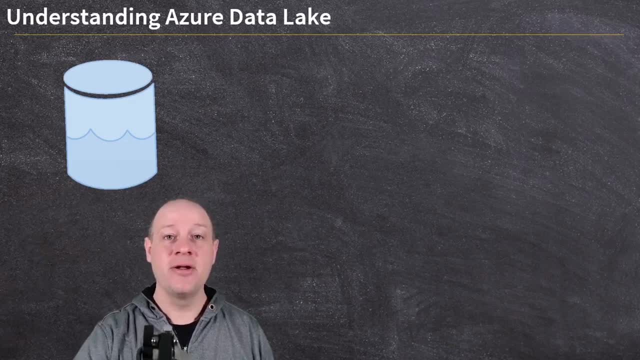 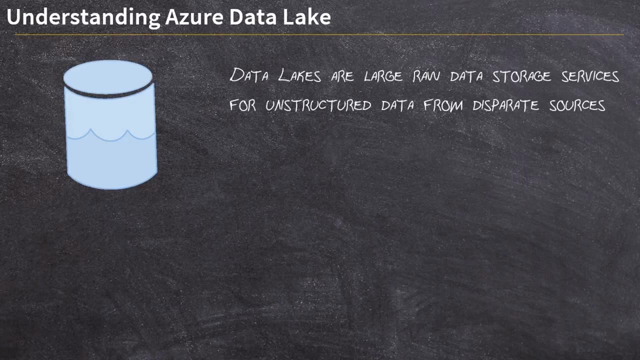 we need a way to collect and store all of this data and enter the concept of a data lake. A data lake is effectively a large raw data storage service And it's for unstructured data that comes from many disparate sources. I want to talk about that first. That's what I. 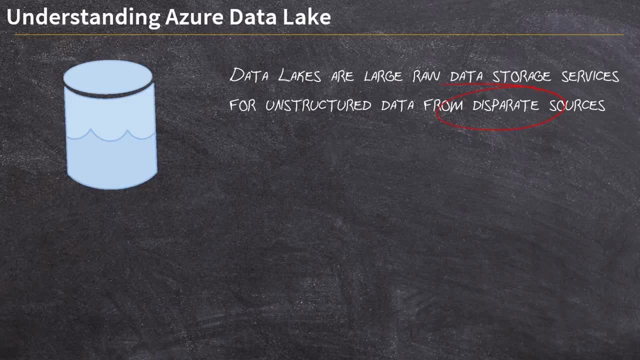 was talking about with regards to the different places that we are collecting data from. It's no longer this highly structured, well-formed input mechanism for data. We're getting all kinds of data from lots of different things that are going to send it in lots of different ways They may. 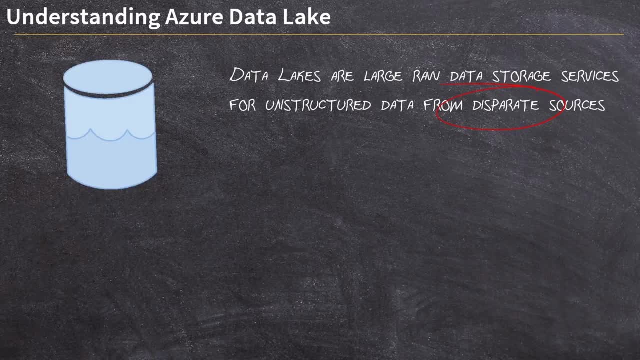 be sending it in raw streams. They may be sending it in JSON or XML. Some systems may be performing a lot of pre-validation. Some systems may be doing no validation. The data may have gaps in it. It may be doubled up or duplicated. The idea with a data lake is that we don't care about any of that. 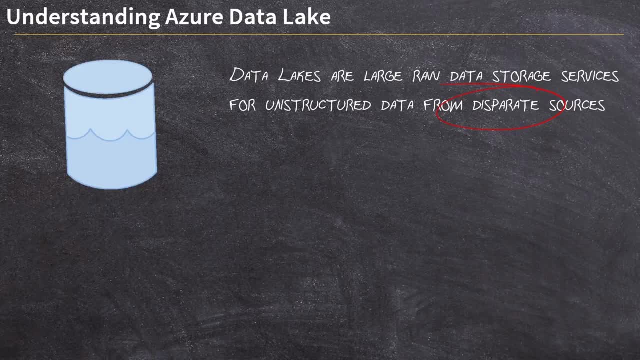 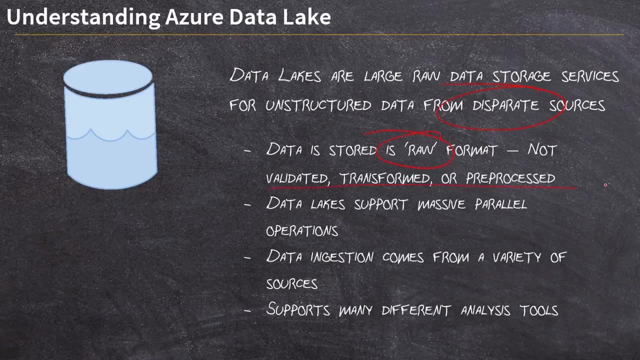 We can collect it all and get it into one. The data lake doesn't care about that. It doesn't validate, transform or pre-process any of that data. It provides a very basic structure, which we'll talk about, in order to store that data, and 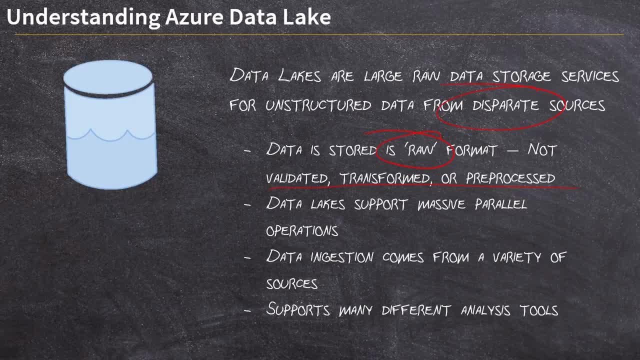 make it accessible And then it's done. The data lake is the storage. It is like a bunch of different streams feeding a lake, just a huge place where you store all of this stuff. What's great about data lakes is they support this idea of really massive parallel operations Once you. 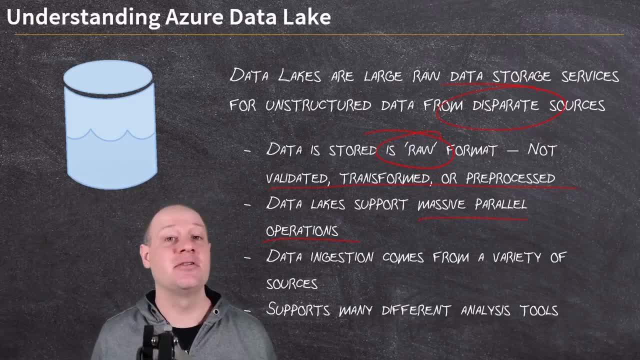 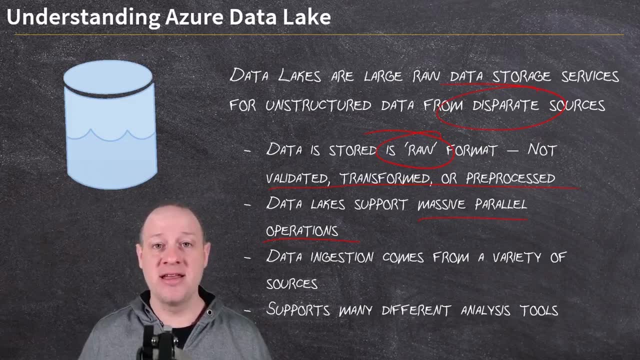 have this data, the ability to actually query that data is going to be computationally heavy, So you need the ability not just to store that data but the ability to run operations against it in a computing-efficient manner. Massive parallel operations are exactly that. They allow you to query the 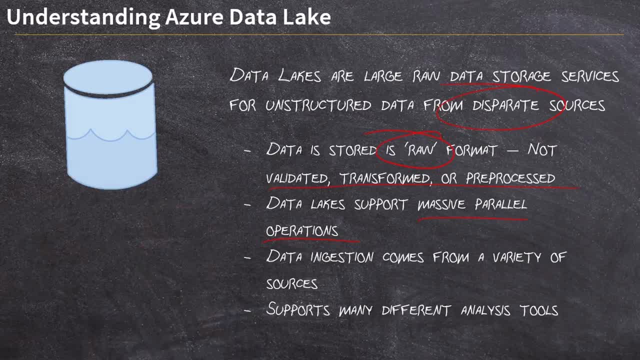 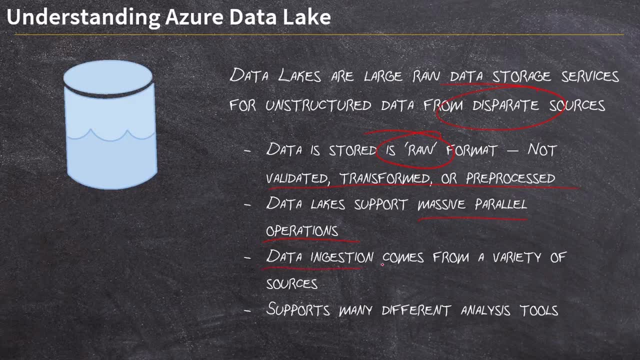 data in parallel and perform these operations and get your answers out of it relatively quickly, at least relative to the size and volume of data. You can also, like we talked about, handle data ingestion from a variety of different sources. When we talk about Azure Data Lake, we're going to 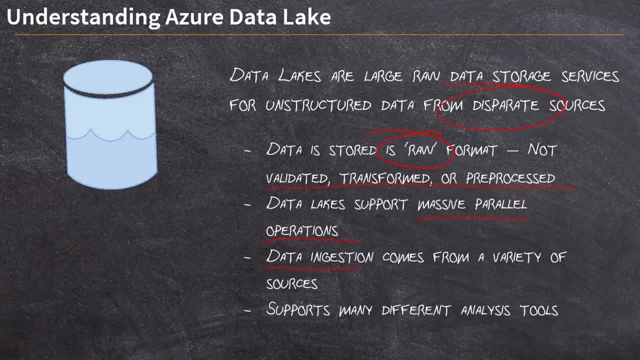 talk about Azure Data Factory for that, but I'll talk about that in another video. And then the output: having all this data inside of your data lake is fine, but you need a way to look at it. So data lakes support a lot of different analysis tools. You need a lot of different ways to. 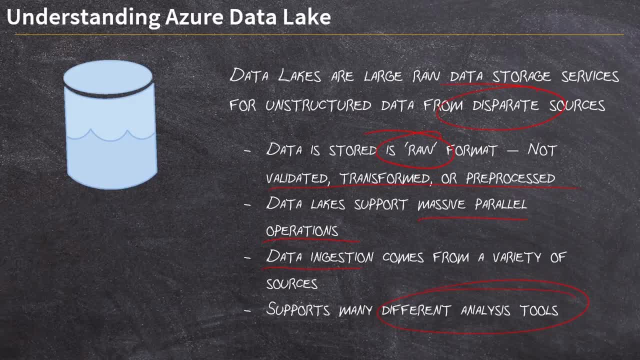 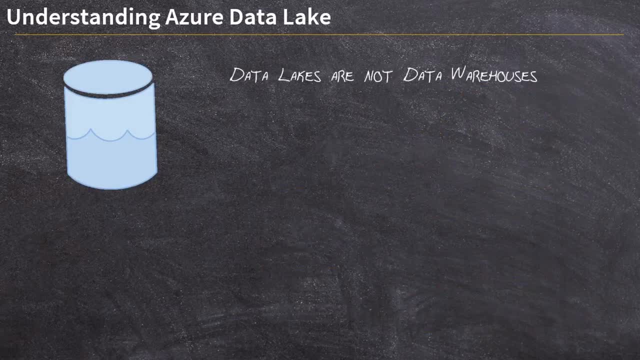 actually look at and understand and gain insights from your data. So one thing that a data lake may sound similar to is a data warehouse. but I want to be perfectly clear: Data lakes are not data warehouses. These are two very, very different things. Data lakes have no real defined reason. 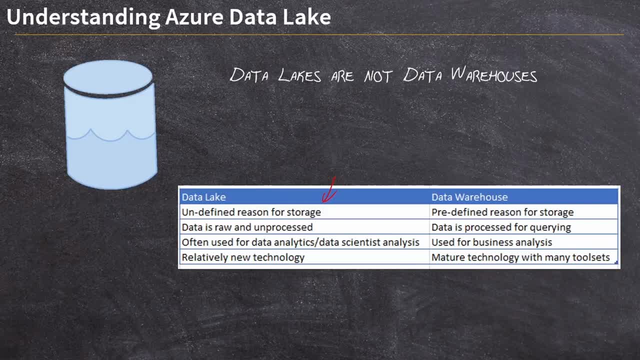 to be stored. Data lakes are not data warehouses. Data lakes are just storage for data. Data lakes are not data warehouses. Data lakes are just storage for data. Data lakes are just storage for data. Let's just get this data in. we'll figure out why we want to look at this data and whether or not. 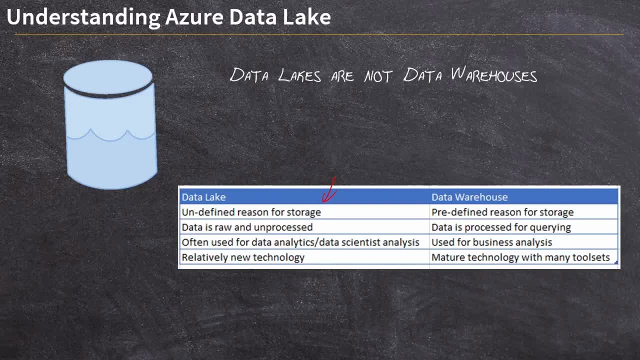 we need it at a future point in time, But for now, we don't want to throw out any data that we're collecting, So let's get it in somewhere. A data warehouse, on the other hand, usually has a fairly predefined reason for storage. With a data warehouse, you are saying: Hey, you know what? 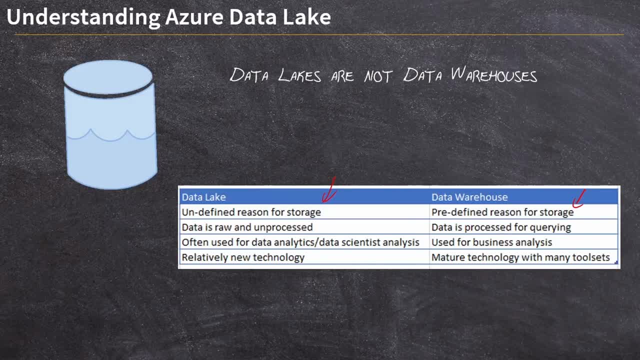 Get this data in this specific data for this specific purpose, so we can run these reports. We can generate this information out of it on a routine basis. yada, yada, yada. Like I said, data lake data is often raw and unprocessed. We don't do a whole lot with the data lake data. 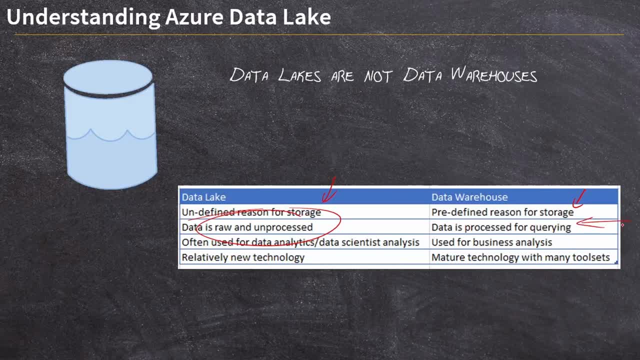 whereas data warehouse data is frequently pre-processed and heavily structured so that we can easily query against it for known business analysis. That's what we want to do with the data warehouse. We're saying, hey, what were our weekly sales this week? Or who was the top volume seller? 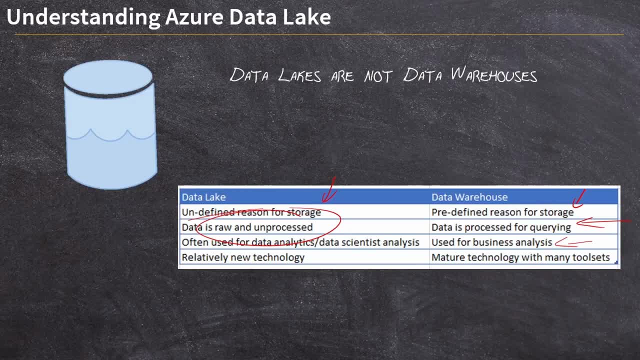 from the past quarter. That sort of thing Data lakes, on the other hand, are often used for things like data analytics and data science. right, ML, think machine learning. They don't care so much about the structure of the data, They just need to have access to as much of it. 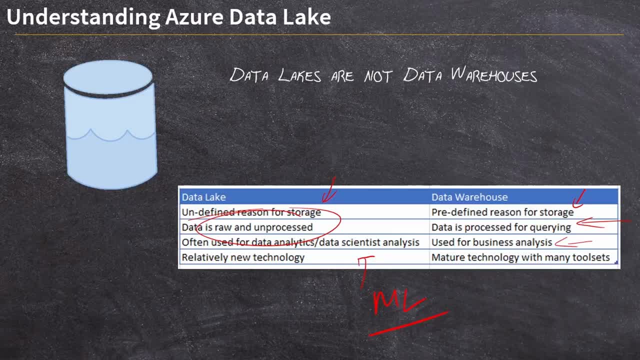 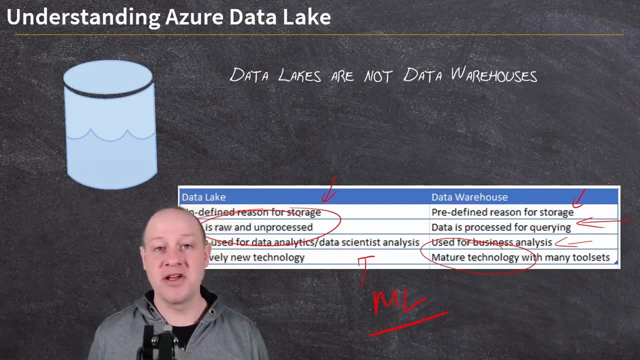 as possible in order to gain insights out of it. Data warehouses are also a very mature technology at this point. We've been using data warehouses for a number of years in the field of data professionals. Data lakes, on the other hand, are relatively new because, like I talked about, 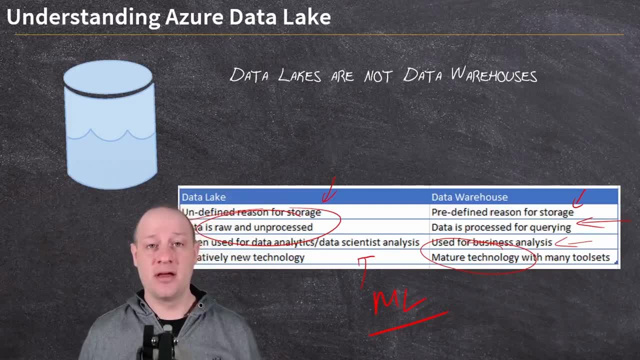 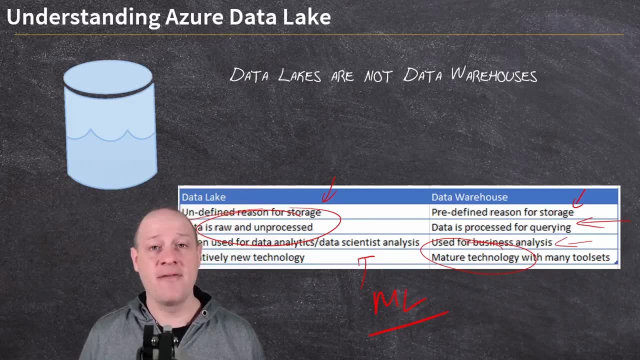 the collection of all this data and the ability to easily store it is really kind of a new thing for all of us. The idea of a data lake and the technology surrounding it are still pretty new. It's pretty bleeding edge stuff even today. So you're going to find that the tool sets are not nearly as mature. There's a lot of different. 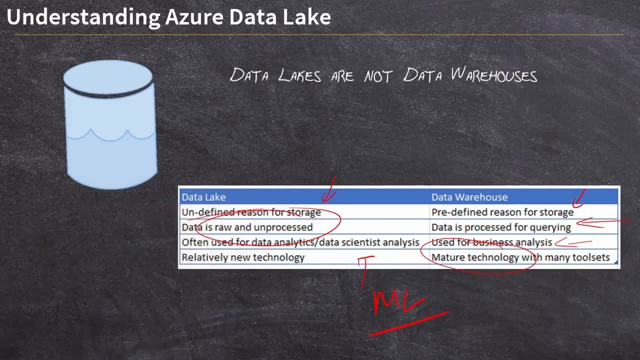 options out there, and some of the standards are not necessarily as well defined as they would be with data warehousing. Now, data lakes are certainly not a concept that is unique to Azure. You're going to find that every major cloud provider has a data lake of some sort. Azure has. 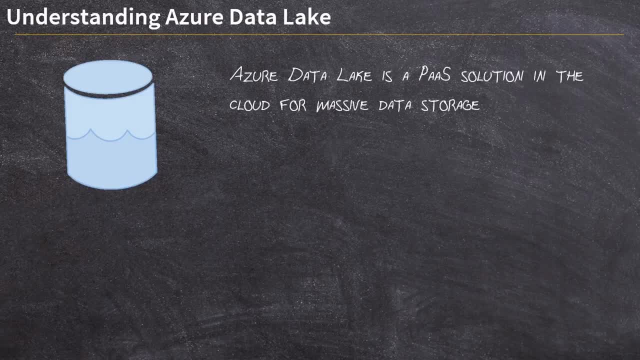 one that they call helpfully Azure Data Lake. So that's literally the name of their service, the Azure Data Lake. It is a platform as a service solution inside of the Azure cloud that allows for storage Some of the features specifically of Azure Data Lake. well, it can support trillions of 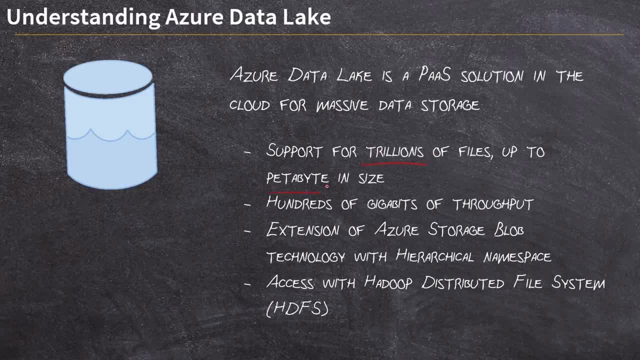 different files, and those files can be petabyte in size. This is effectively limitless. I mean, this is not technically infinite, but it may as well be infinite. Almost none of us are going to run up against any sort of limits, So we can pour as much data into that data lake as we want. 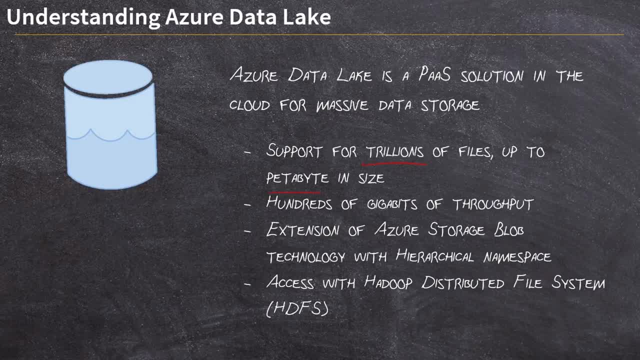 without having to worry about artificial resource constraints on the volume of data. We also get hundreds of gigabits of throughput with that massively parallel processing engine that I talked about. You don't have to worry about queries. You don't have to worry about queries. 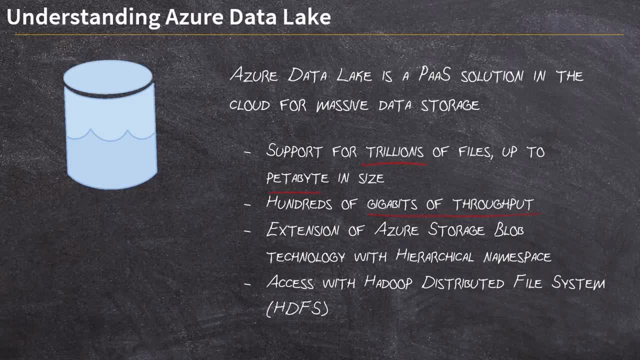 You're going to get very fast, very efficient access to it. It's an extension of Azure Blob technology And this is really, really important. I think I want to talk about this for just a moment. It is truly Azure storage, And when I show you in a minute how we fire up an Azure Data Lake. 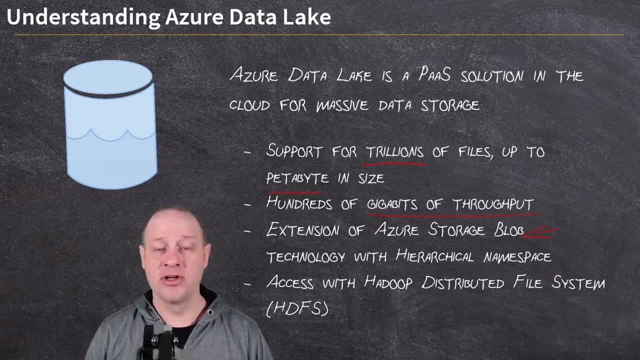 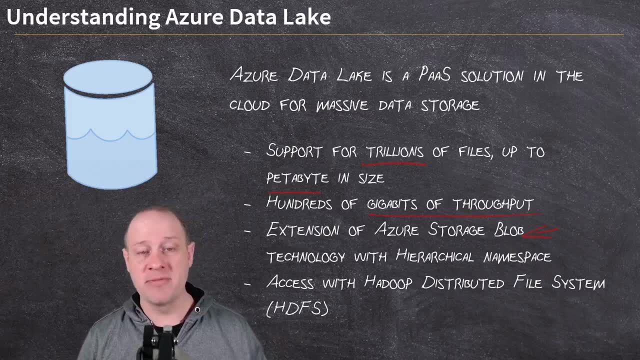 service. you do so actually through the Azure Data Storage interface. It is an extension of Azure Blob storage and it comes with everything that comes with Azure Blob storage. If you watch my videos on Blob storage, you recall that Blob storage, for instance, has: 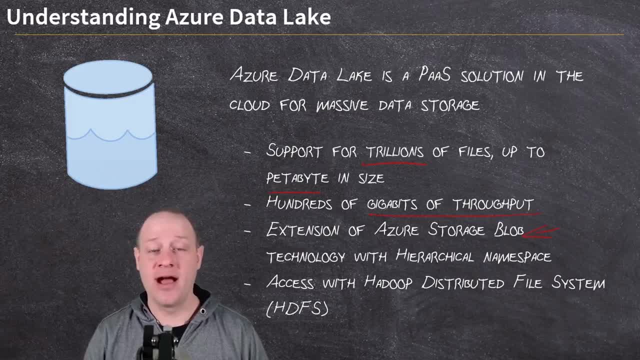 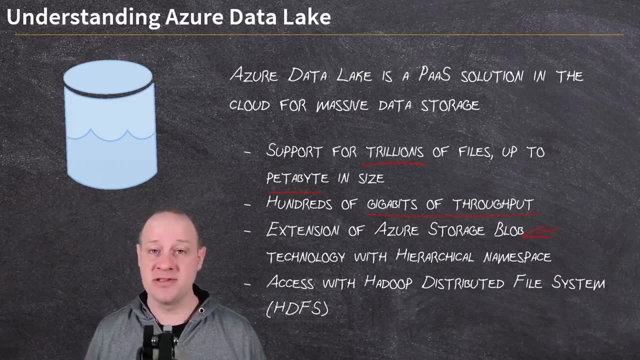 the ability to store access tiers. You have hot, cold and archival. That's available for your data lake as well. It's all secured through RBAC in the Azure IAM identity and access management services. Same thing for data lake storage. You even have your choice between standard and premium. 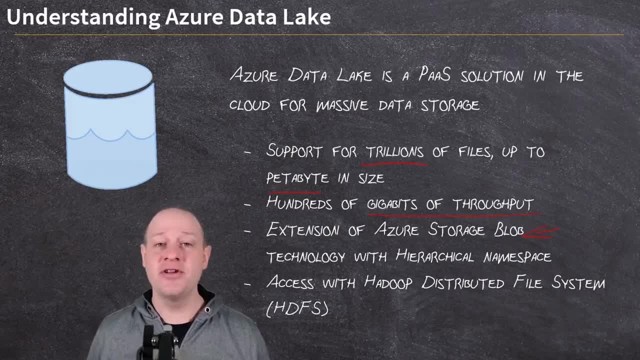 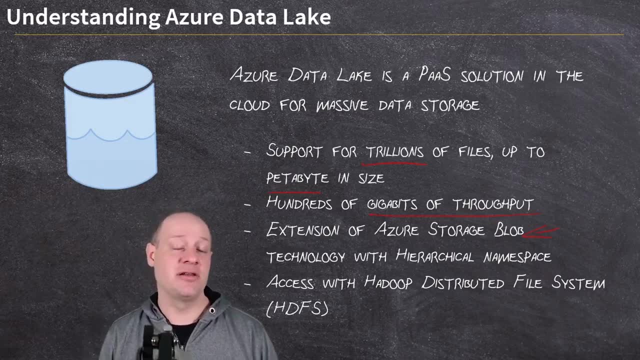 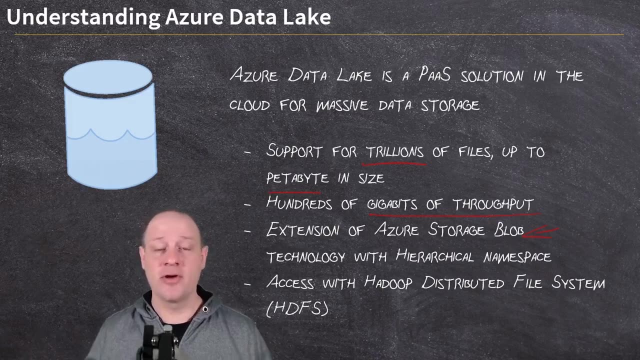 storage. So hard disk drive versus SSD, All of the features, all the functionality that you would expect in Blob storage you also have inside of your Azure Data Lake. On top of that, it layers on something known as a hierarchical namespace- This is well a fancy word for directories, or 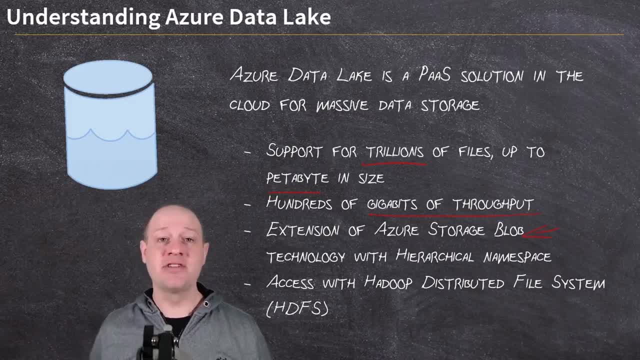 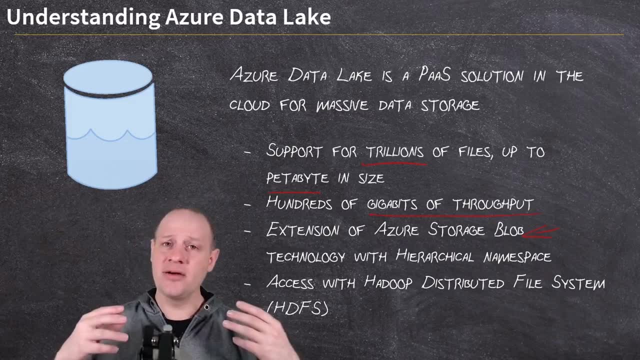 folder names As it stands, with Blob storage. Blobs get stored in containers and that is the extent of the hierarchy. That is the structure that you get. You don't have any folders within those containers. Now you can simulate folders through the Blob name, the entity name, by simply. 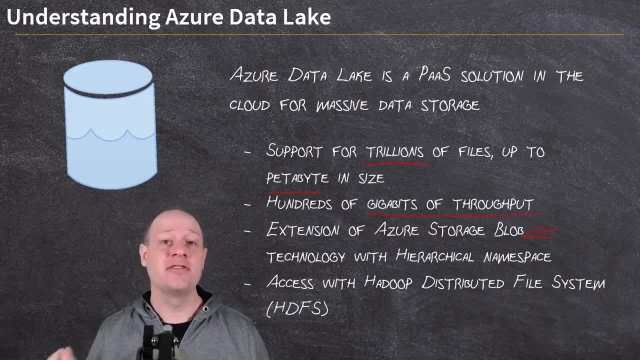 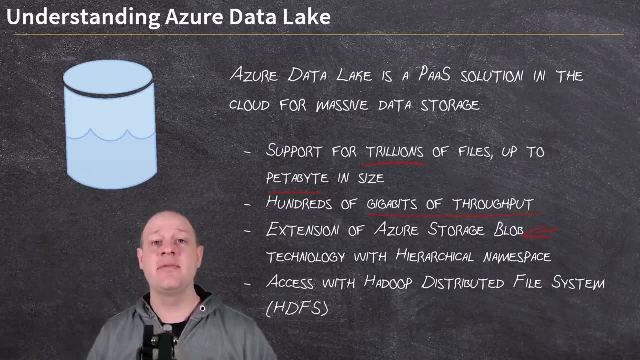 using backslashes or forward slashes inside of the name And that would cause it to look like a folder, look like the Blob belonged to a folder, Particularly in RESTful API calls. you would see those slashes Inside of the name and it would appear like you were divvying it up into folders, even though 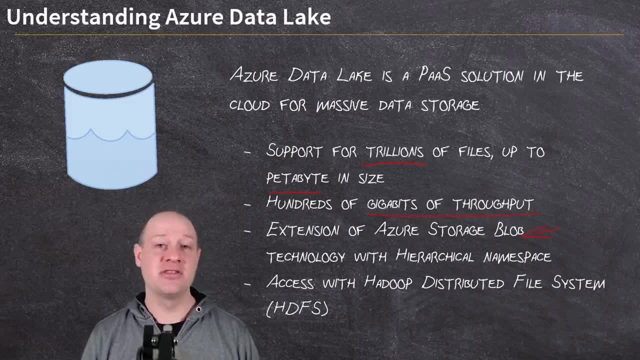 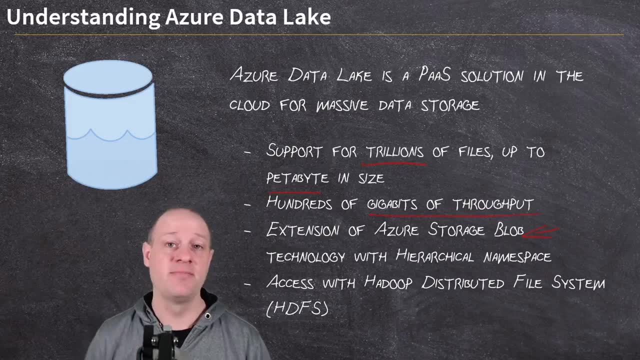 you're really not And the way you know that you're not, you can't perform any operations against that folder. You couldn't delete an entire folder of Blobs because those folders don't really exist. It's just a naming convention, a standard that you are enforcing on those Blobs. 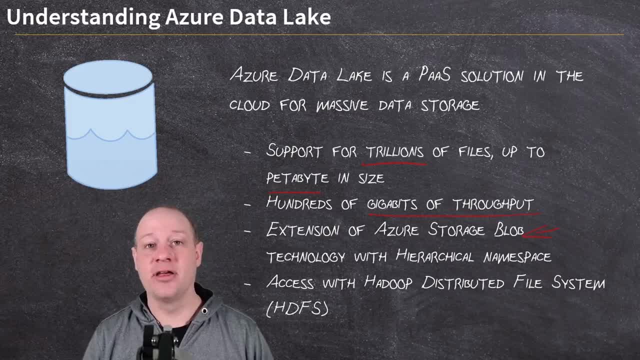 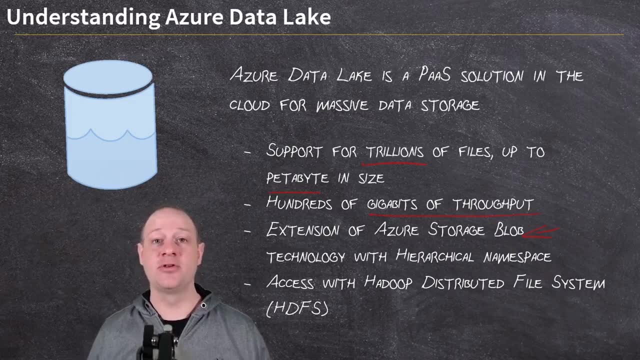 Not so for Azure Data Lake. Azure Data Lake actually has a hierarchy, a folder structure that you can enable, which allows you to perform atomic operations against those actual folder entities, those folder objects. So you can rename an entire folder, You can delete an entire folder. 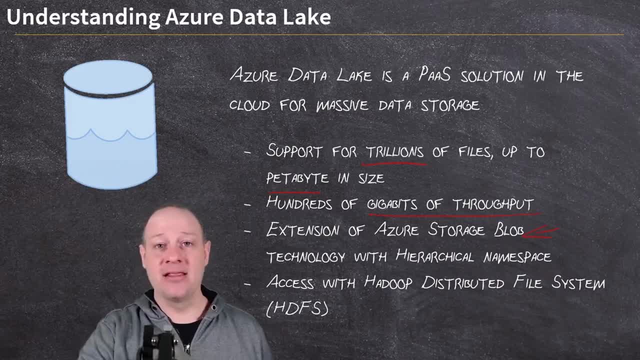 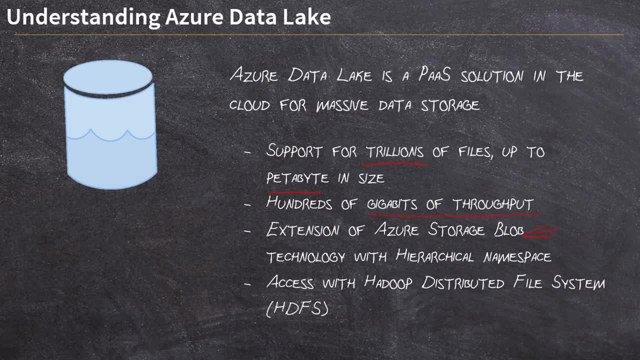 with a simple operation. You have access to your data at that level, which does not exist in Azure Blob storage. You also have access to security at that level, So your security can be applied both at the entity level, the object level, inside of Azure Data Lake, as well as at that folder. 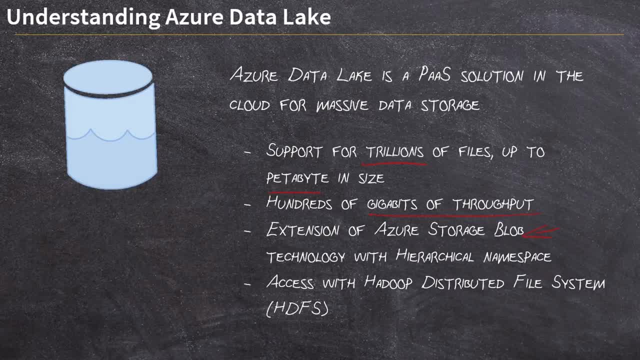 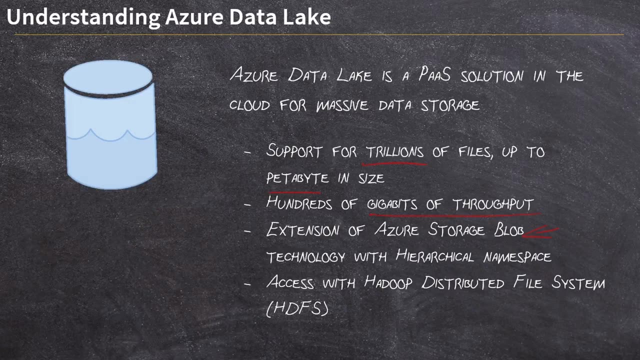 structure level. You can apply access control lists, ACLs, You can apply IAM and RBAC to those things. So you have this actual entity, this actual structure that supports both your operations as well as your security at that level, inside of the container, that does not exist for standard Azure Blob storage. 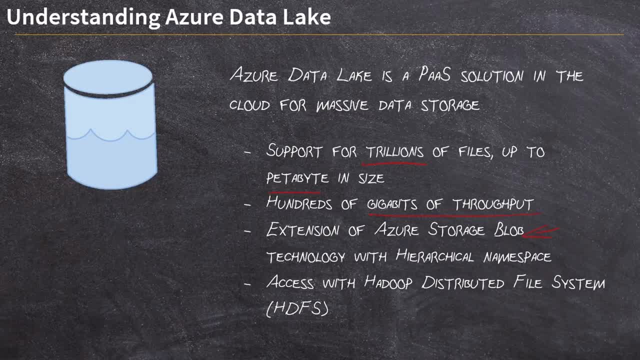 Lastly, your Data Lake is accessed with the HDFS Hadoop Distributed File System. All modern implementations of the HDFS have the appropriate protocols for interacting with your Azure Data Lake. Hadoop is an industry standard for big data analytics, So if you are in the 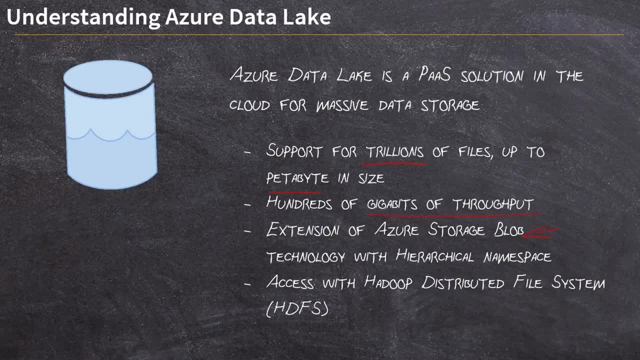 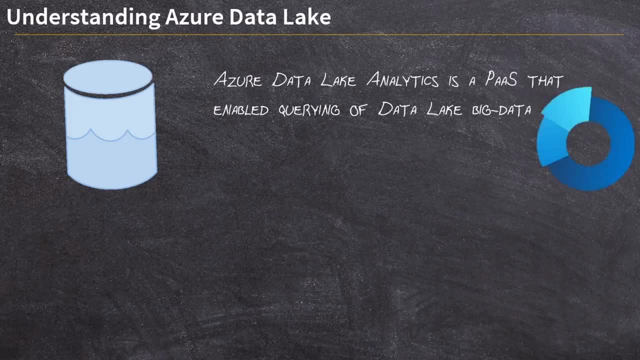 world of Data Lakes and big data. you should be familiar with Hadoop. Now, Azure Data Lake also has a couple of additional components to it. One is called Azure Data Lake, which is a data lake analytics, And Azure Data Lake analytics, like the name might imply, is an analytics. 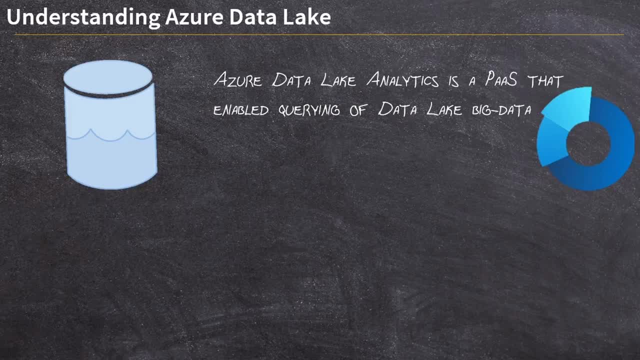 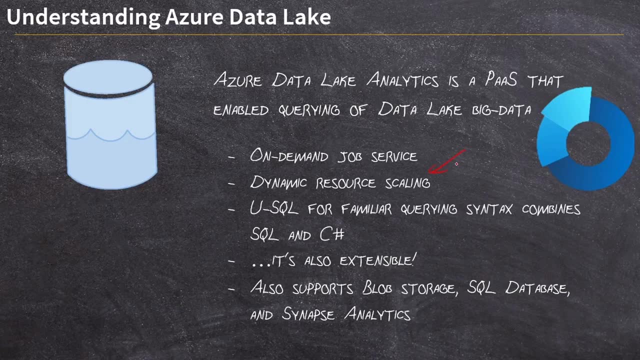 service for Azure Data Lake. It allows you to query your Data Lake big data very, very easily. It's an on-demand job service with dynamic resource scaling. What does that mean? That means you don't have to provision a server to run it. You don't have to worry about RAM or CPU. 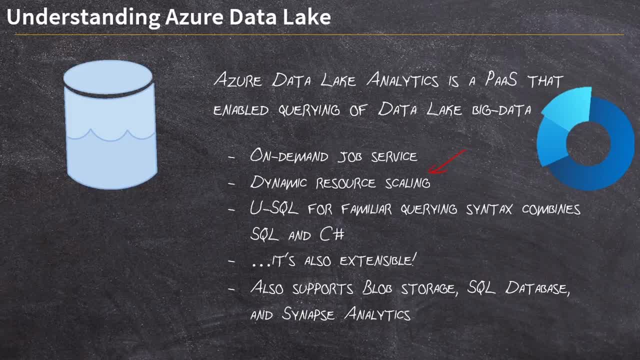 requirements. You simply set up and create your jobs, and Azure will handle scaling up and scaling down resources in order to support the querying job that you want to run. And, speaking of those queries, it uses something called USQL, which, yeah, like you guessed, it is really just. 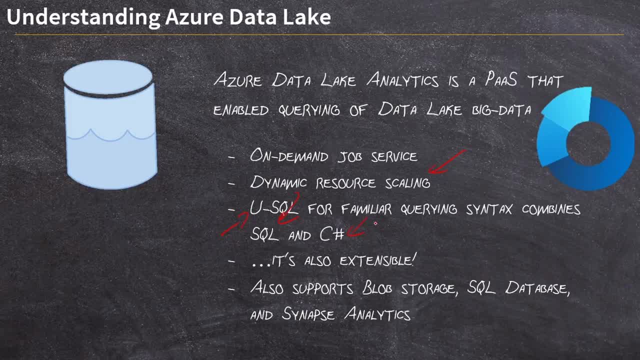 an SQL syntax, although it combines it with C-sharp. So database developers and programmers- C-sharp developers- are going to be very, very familiar with how to use this query in order to support querying and reading data out of your Data Lake with Data Lake analytics. It's also 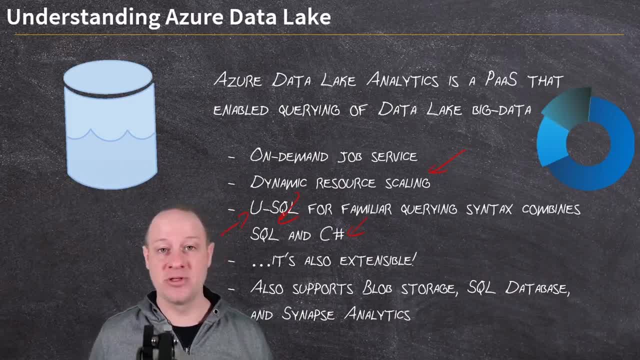 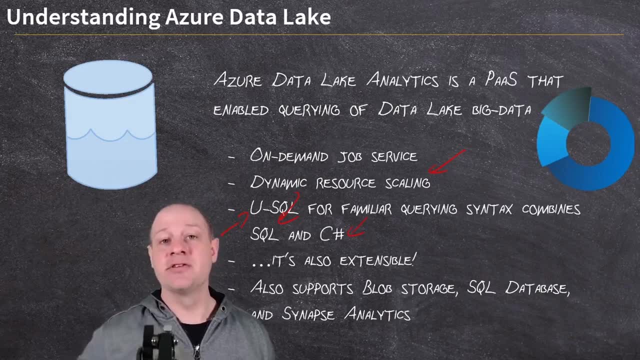 extensible Because it's running C-sharp. you can build additional modules and additional code for yourself on top of it and extend the language and the capabilities to you know your specific needs, which I think is pretty cool. So it's not just SQL and C-sharp. 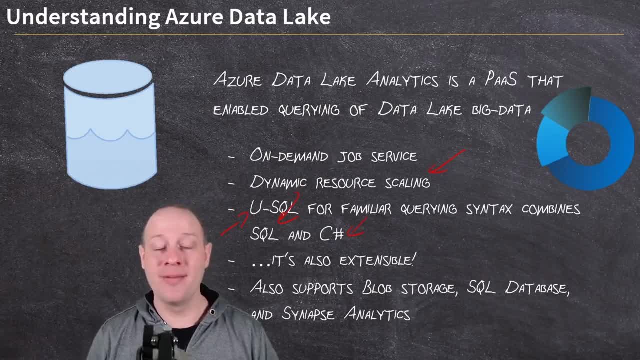 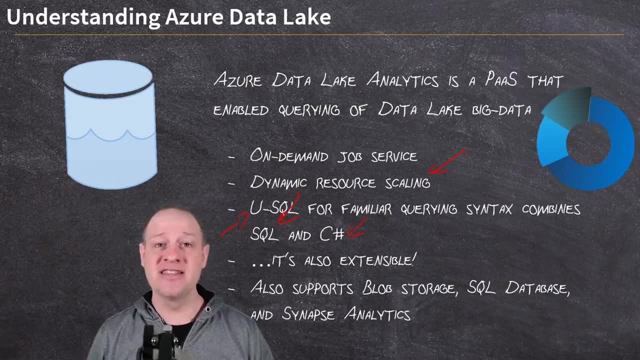 combined, It also brings in all of the power of development and programming in the NET platform, including the ability to integrate with Visual Studio. If you're a developer, a NET developer, you know what Visual Studio is. That's where you develop your NET code. Azure Data Lake analytics. 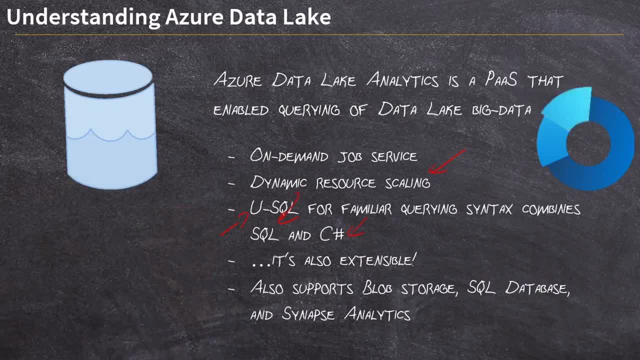 integrates directly with that, so that you can write your code and you can write your USQL right inside of your existing tool set. Now Azure Data Lake analytics is cool because it doesn't just support Azure Data Lake, It also, of course, supports blob storage. 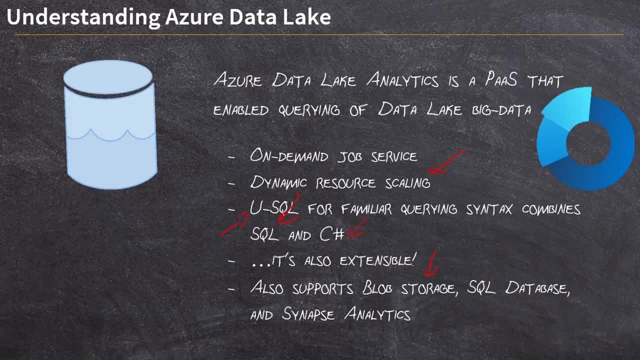 Because, at the end of the day, Data Lake is blob storage, But it also supports Azure SQL database. That's the SQL PaaS solution and something known as Synapse Analytics, which we will talk about in another video. So Data Lake analytics supports all of these things. It doesn't.